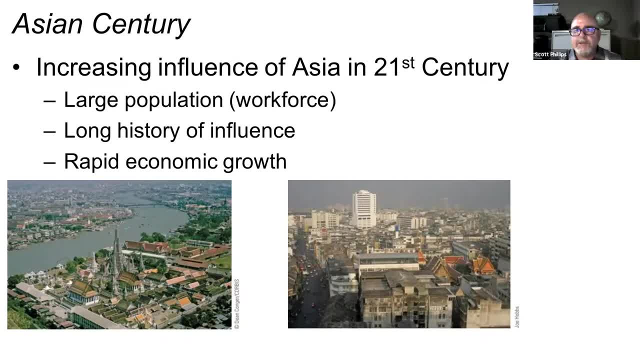 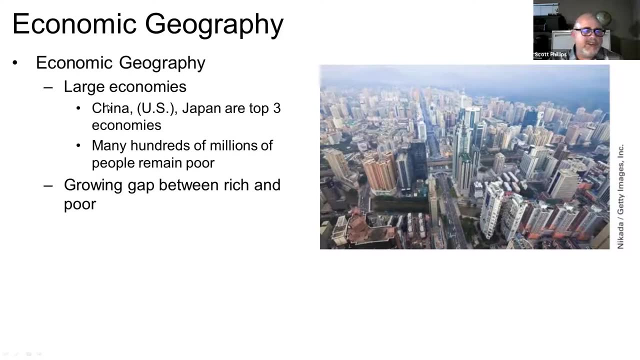 And in recent times it's really catching up quickly in terms of economic growth. It's like the Industrial Revolution, but just super fast. This happened in East Asia, So it has large economies, And the three largest economies in the world are China, the United States and Japan, So in East Asia we have two of the three largest economies. 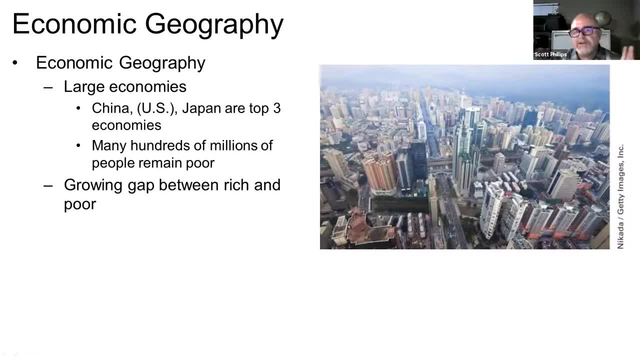 And in some way China and the US are pretty close to each other in terms of their- depending on how you measure it- the size of their economies, But there's still a lot of poverty as well, especially in the rural areas. So it's not always evenly. the growth isn't always even. A lot of it has been concentrated in some of the kind of high growth areas of China. 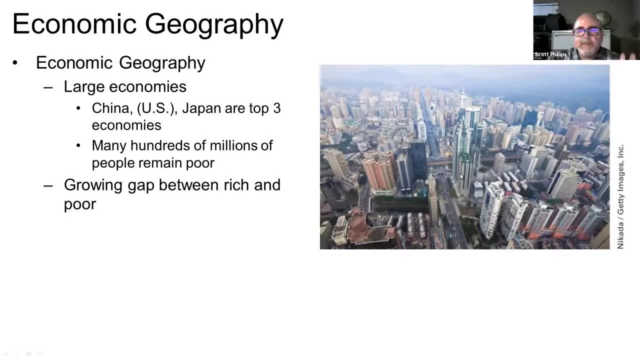 And where there's a lot of money. there's a lot of money that's being developed because of all the industry in China, But there's a bigger gap growing between the rich and the poor, especially in the poor Rural areas, And that gap helps to kind of draw in people into the urban areas. 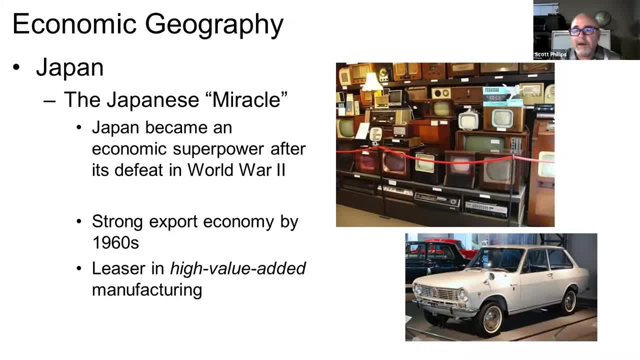 But well, if we want to look at the growth of the economies in East Asia, we have to start with Japan, because Japan was a fairly industrialized country prior to World War II. You know, I mean it was big enough that it challenged, you know. you know we fought them. the United States and Japan were locked in. 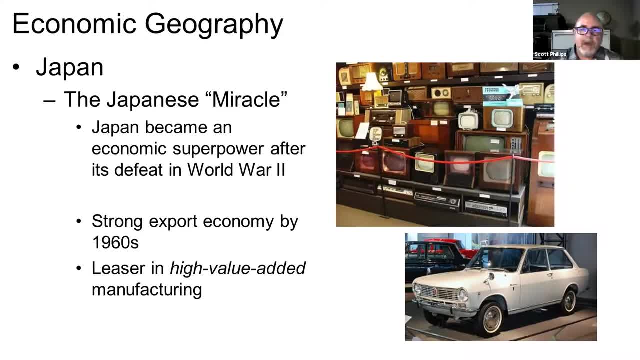 You know, in war during World War II, but the US won. but after the war the US tried to make it an ally because in the Cold War helped them, like with Western Europe, rebuild some of their economy. But their economy really took off like a rocket. It's called the Japanese Miracle and Japan really came right back as an economic superpower after World War II. 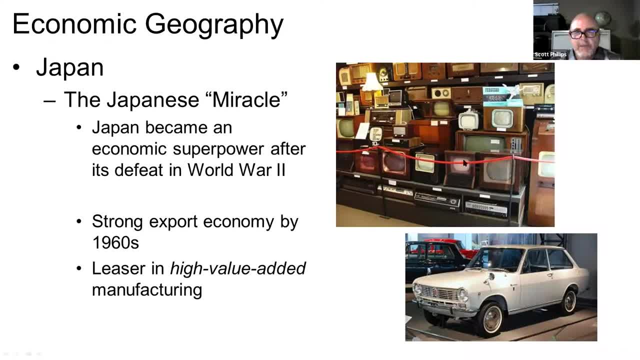 So by the 1960s Japan had a soup, you know, was making a lot of money of products, television, cars. um, if the way we think about, if you think about today, about all of the computer products and phones and things that are made in china, japan used to be that that you know. 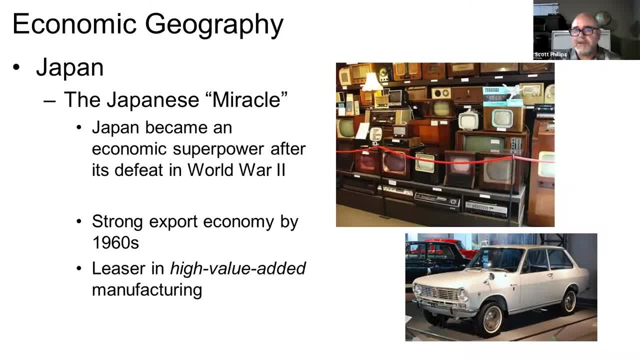 it used to be that people said the same thing about japan that they say about china now, and it still continues. but in japan it's a little different because it's like higher-end products like automobiles, scientific equipment. they are a major producer of this, these types of goods. 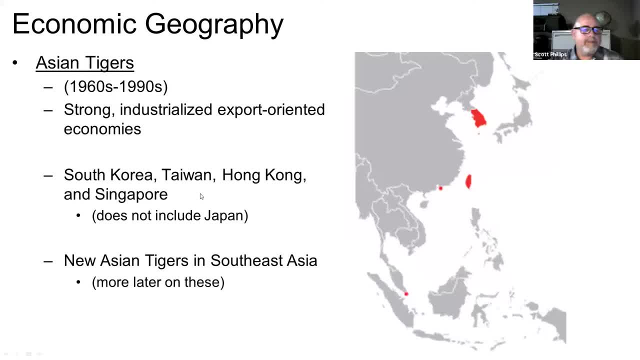 say leader, not leaser. okay, so one, you have japan. after japan you had um four other economies that really can kind of really rocketed um in the 19 in the, you know, from the 60s to the 90s after japan really took off, you had four that kind of came. 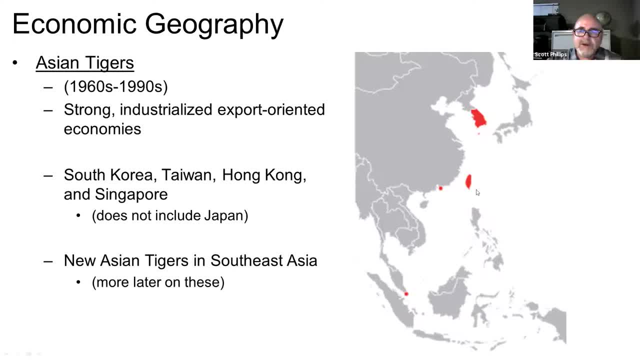 after called the asian tigers. these are strong, industrialized, export-oriented economies, like japan was, so this does not include japan. japan is earlier. therefore there's south korea, there's taiwan, hong kong and singapore. we'll cover singapore more later because it's a little bit outside of the realm, it's in the south. 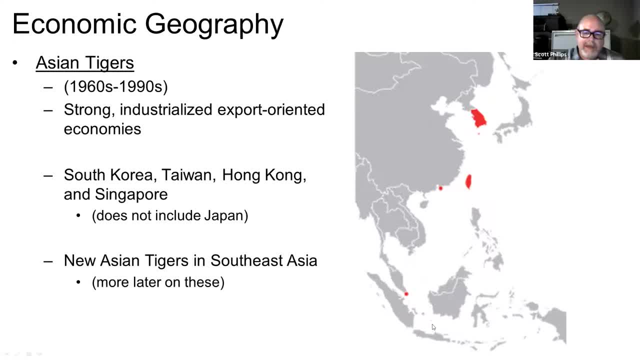 east asian realm and around singapore you have what are called new asian tigers, but we'll talk more about those in the next chapter. say so: you have japan, one, two. you have the tigers right now. at this time, china was lagging behind because it was still under all you know, it was still a. 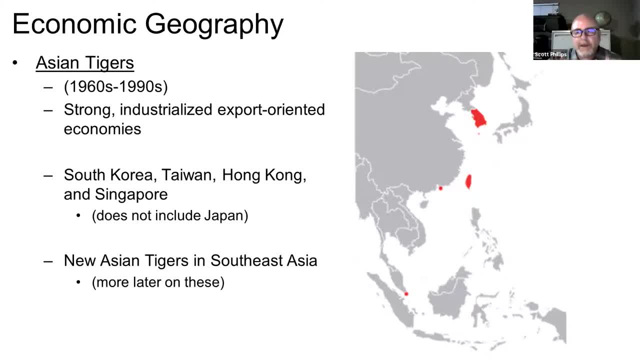 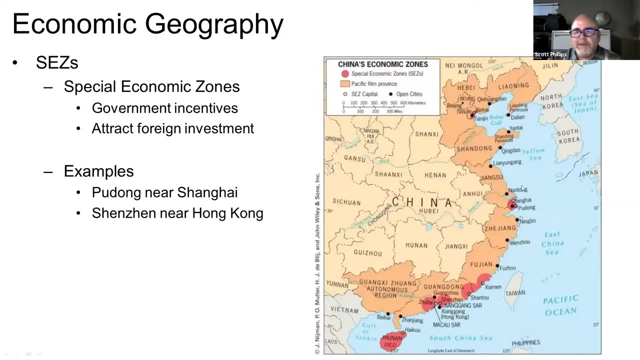 mostly a communist um economic system. however, just off the coast here you had taiwan and hong kong. their economy is really taking off. so the way china's economy developed initially was through special economic zones. um china, seeing you know the growth of these asian tigers, started to set up special zones. 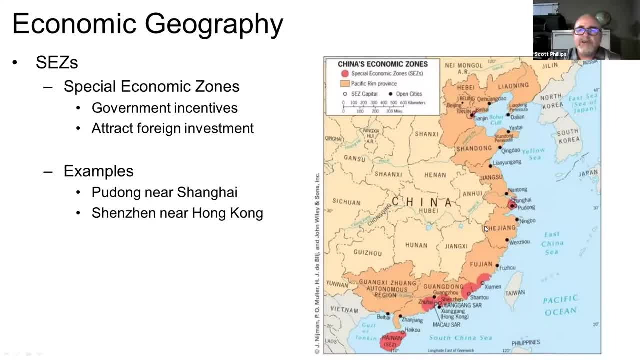 where there was different government regulations to encourage foreign investment. um, the two big ones- and i'll use these as an example- is this pudong one. this is senator wang in china. and then we moved on to fujian. it is in china, right around shanghai. 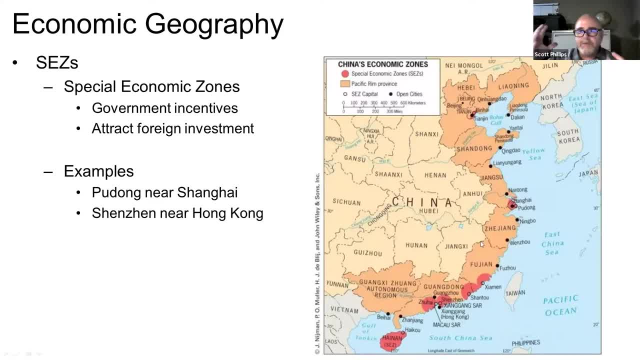 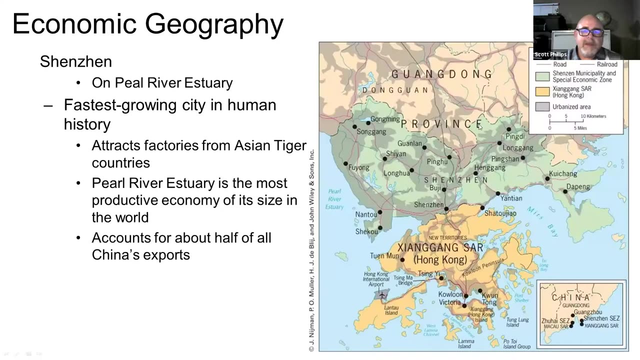 and we have a chinese area called shenzhen which kind of surrounds hong kong, and these are now kind of the two. first hong kong, then shanghai became two big, big economic powerhouses of the chinese economy. let's take a closer look at shenzhen. 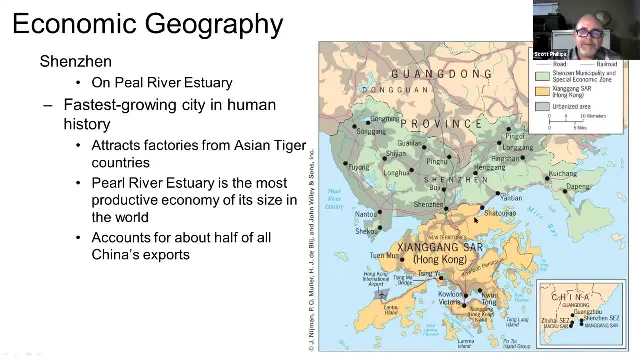 province of China. you have Hong Kong here, so it's like this island. it's a little bit of a separation here and Hong Kong wasn't controlled by China. it was controlled by the British into the 1990s and became an economic powerhouse in this region and over time that this influenced China this kind. 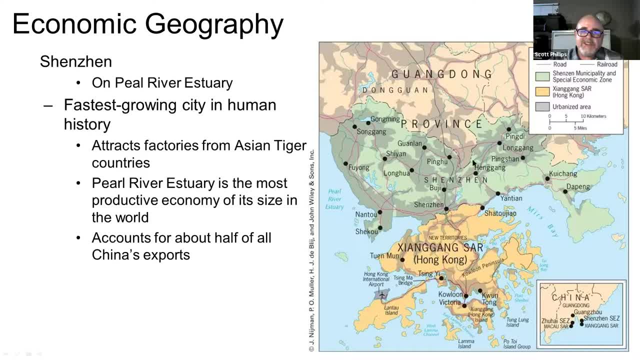 of drew investment from China into the Shenzhen region, which is now- I mean, Shenzhen is like the size of New York City, and that happened within like a decade. this is a rapidly growing part of China. this is where a lot of the high-tech- this is like a super hype- there's like their big tech. 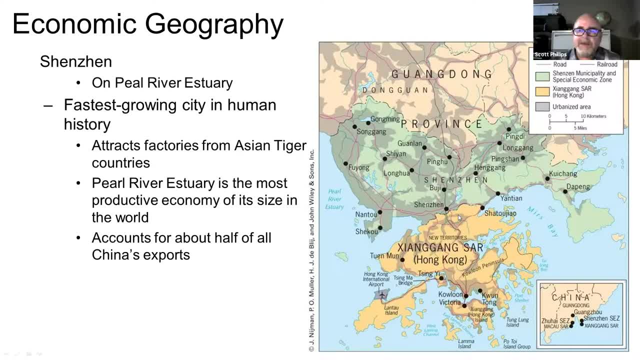 hub right here near Hong Kong, and a lot of that came because of working through Hong Kong initially, and so that's what kind of spurred the growth of the Shenzhen region. so this whole area- this is that Pearl River estuary that influenced Shenzhen and Hong Kong. it's the most productive economy. 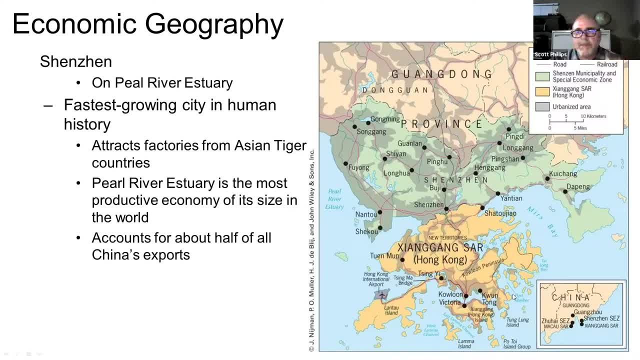 of its size anywhere in the world. this is a super high manufacturing just a lot of money. about half of Chinese exports come from this kind of region of Shenzhen, Hong Kong- and, by the way, just a side note, like I mentioned, the Shenzhen is considered the fastest-growing city in human history. that 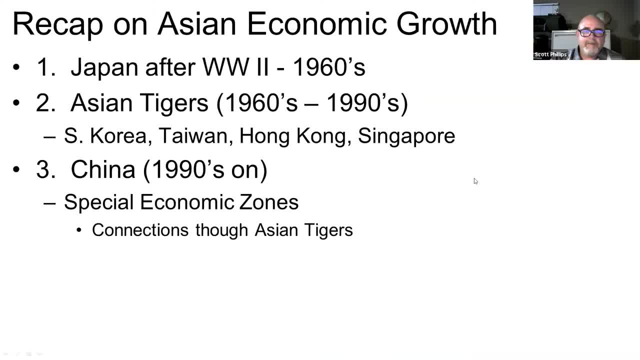 this is really happening at a fast pace. so just to recap, we have Japan, initially, World War II to the 1960s. after Japan we have the Asian Tigers: South Korea, Taiwan, Hong Kong, Singapore and Hong Kong and Taiwan become conduits for trade with China. so because Taiwan and Hong Kong are their close proximity, they 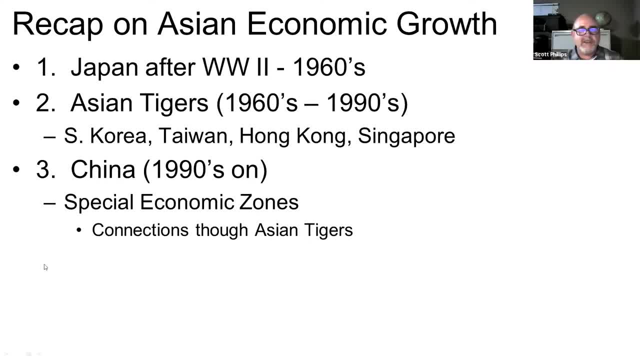 start to kind of tap into the Chinese market. eventually the Chinese kind of take on kind of to this and they become like a tiger. but because they're so big they really surpass the other economies and have really grown to be this one of the biggest, one or two biggest economy.